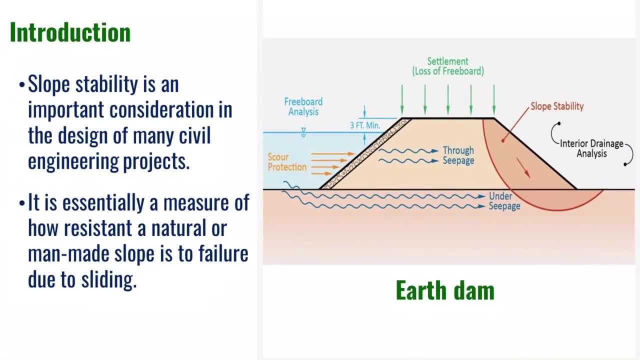 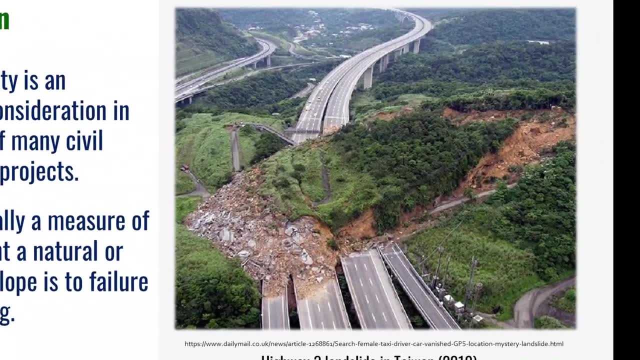 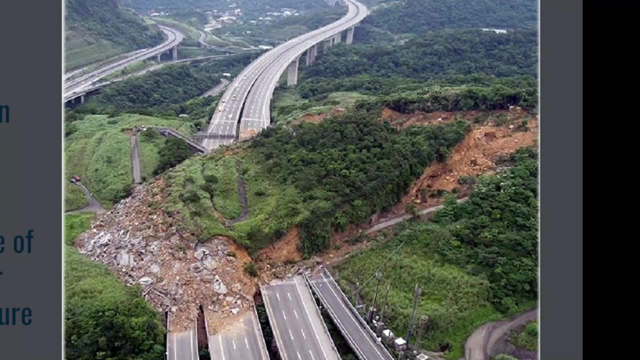 The results of a slope failure can often be catastrophic and could involve loss of property and human lives. What you see here is a disastrous landslide that took place in April 2010 in Taiwan. The landslide destroyed a large section of the land. It caused significant damage to nearby properties. 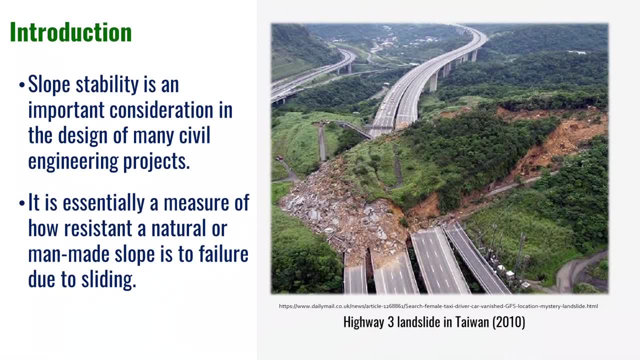 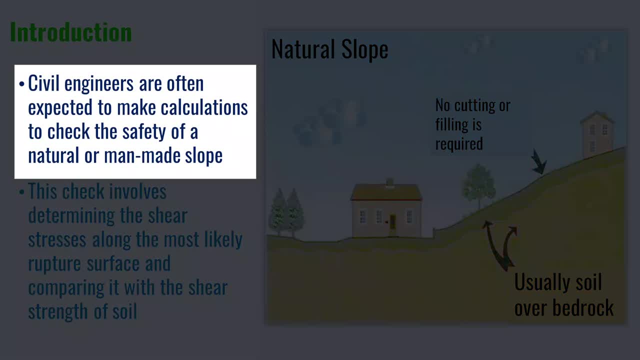 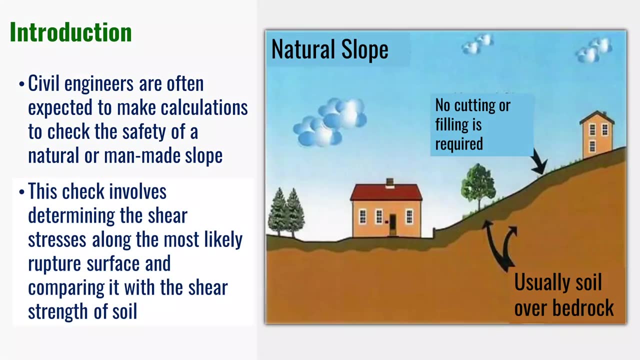 So what is the role of a civil engineer in preventing these types of failures? Well, civil engineers are often expected to make calculations to check the safety of a natural or man-made slope. These calculations usually involve determining the shear stresses along the possible failure surface and comparing it with the shear strength of the slope. 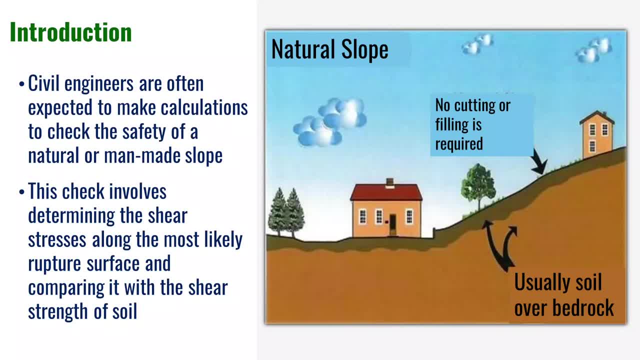 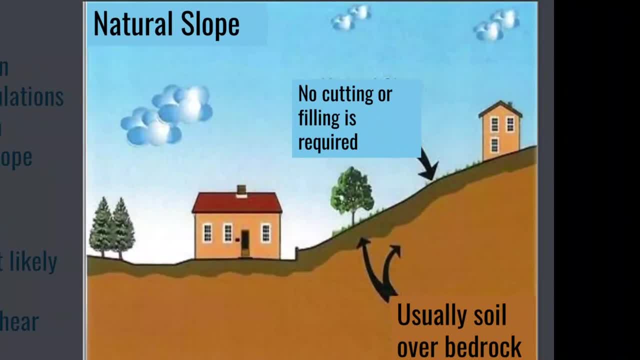 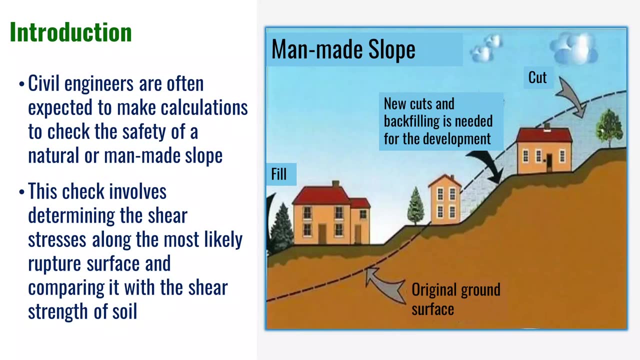 And if you wonder what is the difference between natural and man-made slope, Well, a natural slope is generally unmodified and no material is added or removed from the slope, Whereas man-made slopes can be fully engineered slopes such as earth dams and embankments. 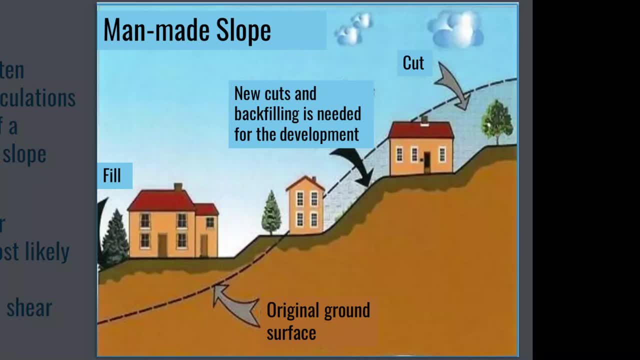 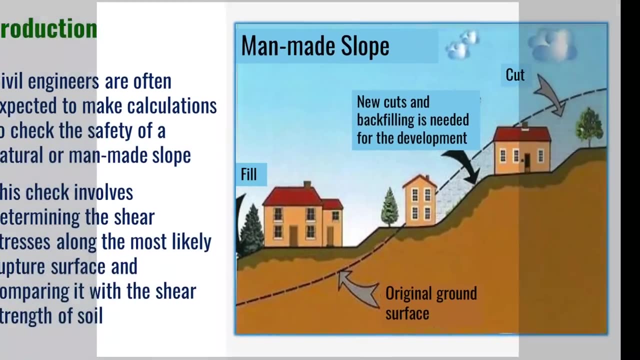 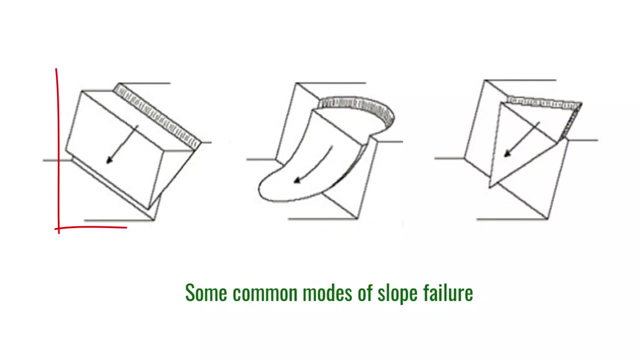 But it also applies to natural slopes that have been significantly modified by cutting and backfilling the areas. Slope failure in soils can take different forms. The most popular ones are translational failure, rotational failure and wedge failure. The failure mode depends heavily on the geology of the slope and the triggering mechanism that led to failure. 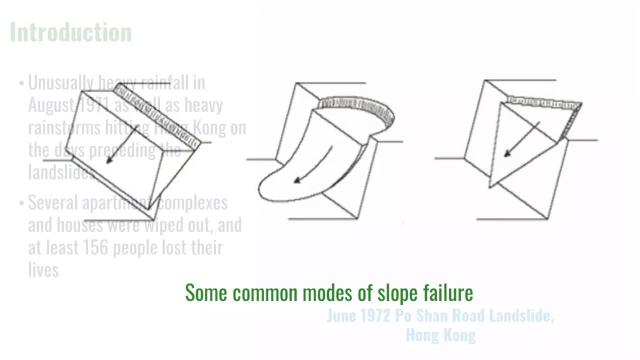 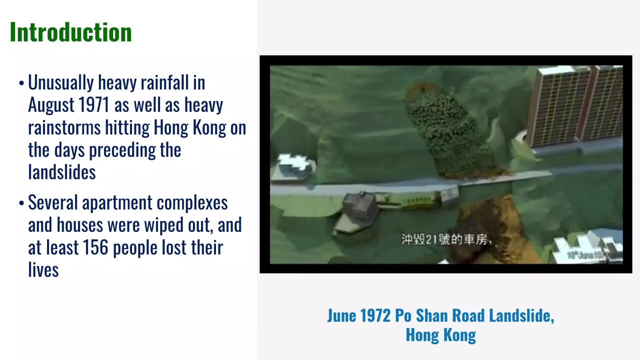 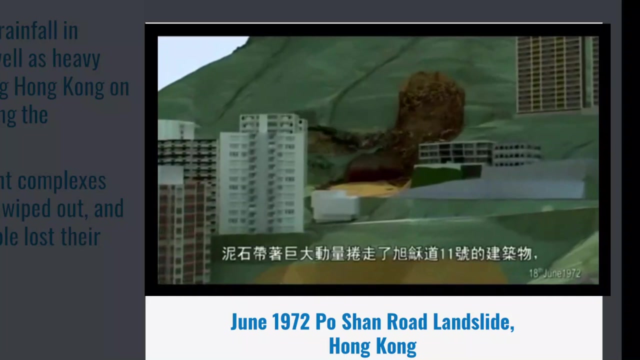 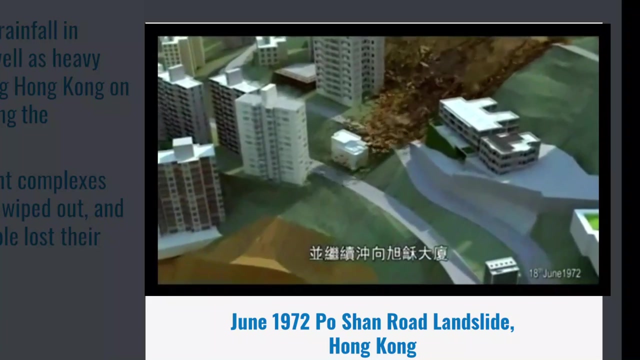 This is a computer simulation of the devastating Proshan Road landslide- Proshan Road landslide that took place in 1972 in Hong Kong. The landslide wiped out several apartment buildings and at least 150 people lost their lives. The site is located in the western med-level area of Hong Kong Island. 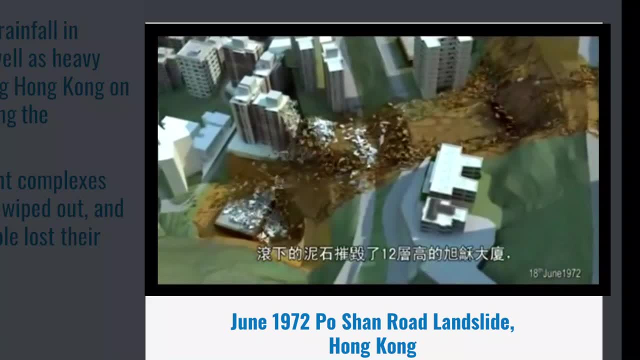 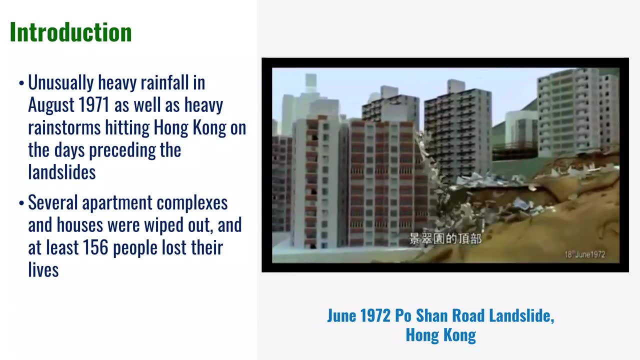 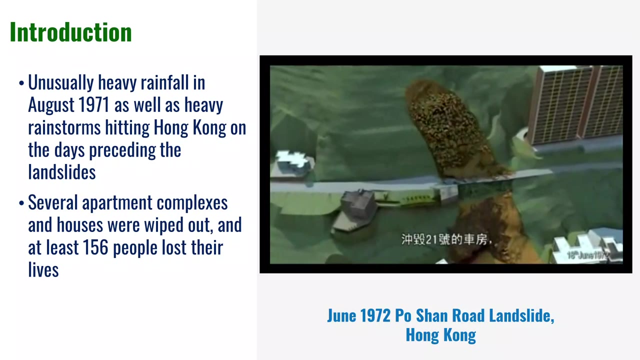 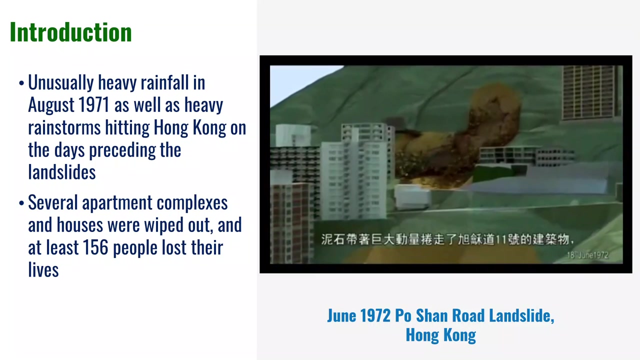 The steep slopes make the site prone to landslides, particularly during heavy rainfall season. Prior to the 1972 disaster, there had been a history of minor landslides and aborted construction activities in the vicinity of this landslide. The rainfall in June 1972 was reported to be almost twice the average and the fifth highest on record. 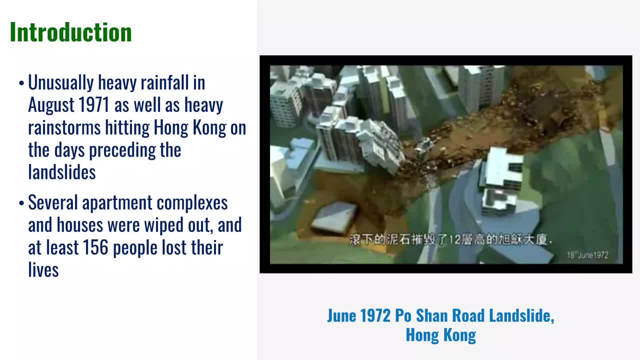 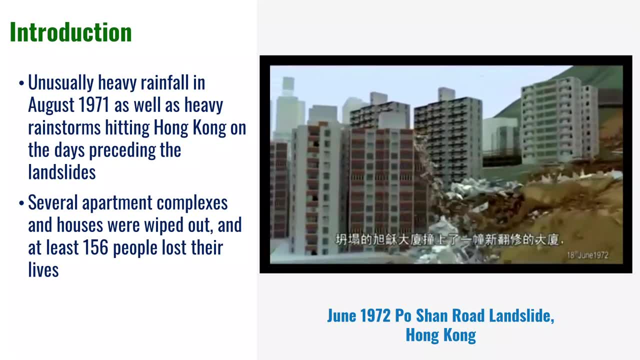 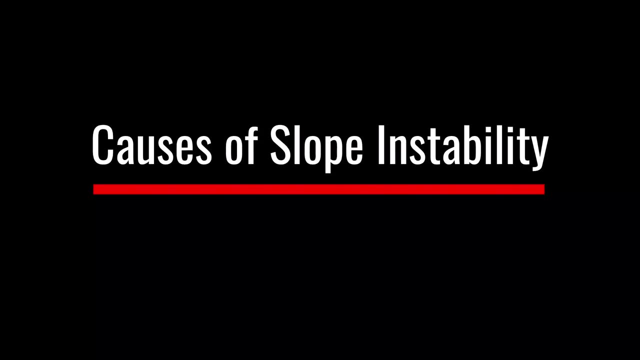 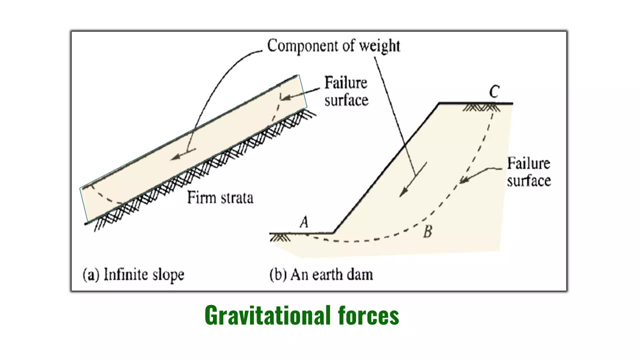 The effect of water on the shear strength of soils was presented in details in episode 2 of this series. Let's now try to understand why slopes fail. The important factors that cause instability of a slope and lead to failure are: First, gravitational force, which is the weight of the slope material in the direction of the failure plane. 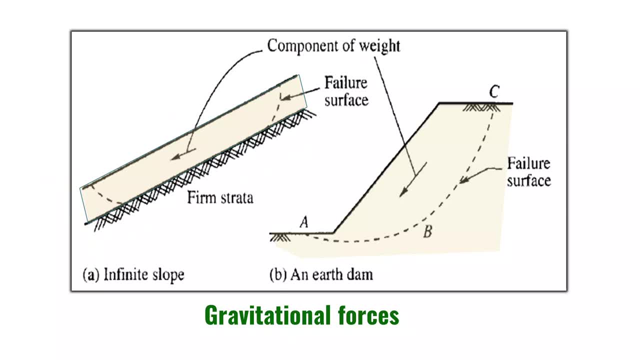 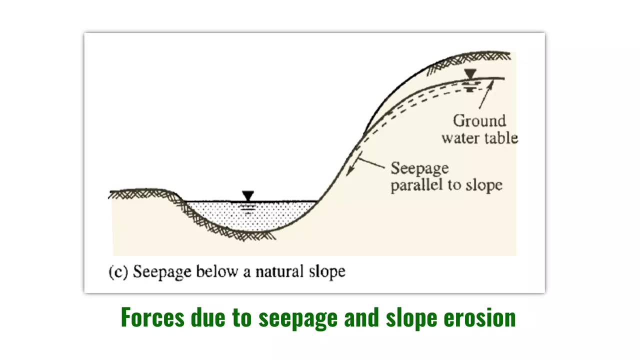 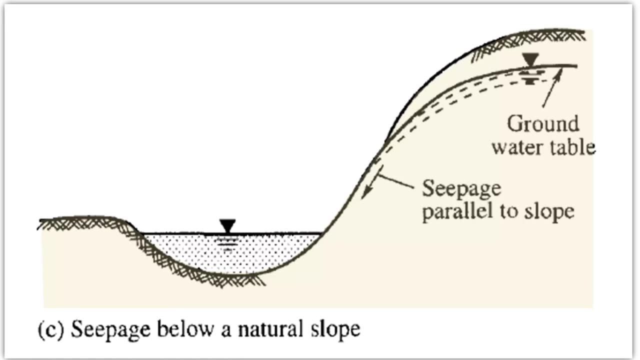 This is applicable to both infinite as well as finite slopes. The effect of seeping water is important in stability problems. Seepage occurring within a soil mass causes seepage forces which have much greater effect on the soil strength as well as particle movement. 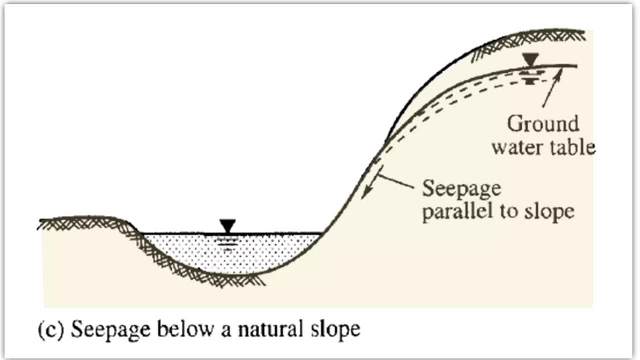 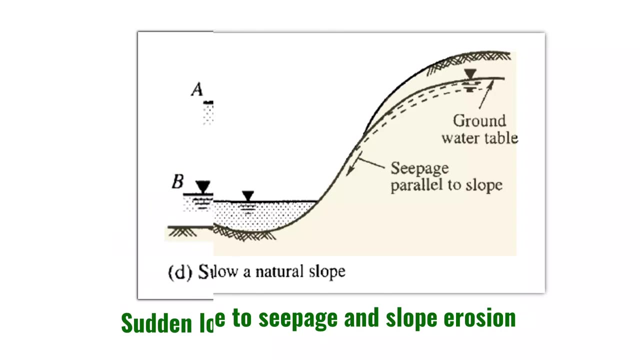 Erosion in the form of undercutting at the toe may increase the height of the slope or decrease the length of the failure surface, And therefore this could lead to a decrease in the stability of the slope When there is a low slope. 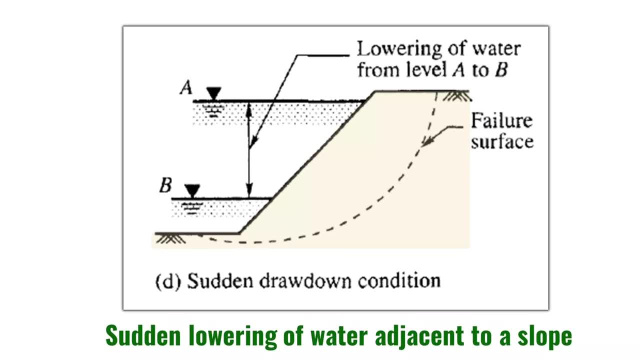 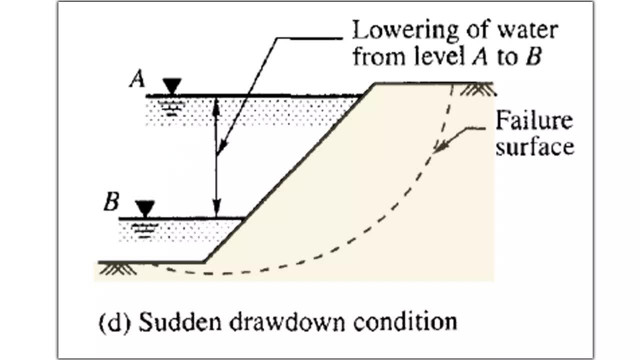 there is a lowering of the free water surface adjacent to a slope, For example in a sudden drawdown in a reservoir. there is a decrease in the buoyancy of the soil which increases the soil weight. This increase in weight causes increase in the shearing stresses. 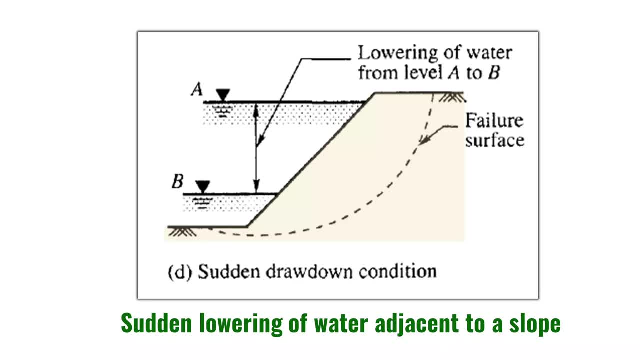 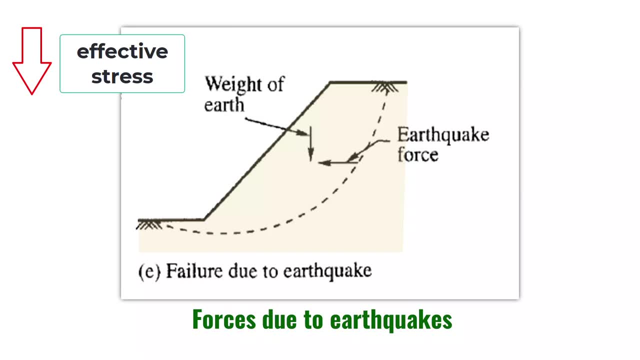 that may not be counterbalanced by the increase in shearing strength, leading to unstable slope. Earthquake can cause a decrease in the intergranular pressure and an increase in the neutral pressure. A failure may be caused by such a condition, in which the entire soil mass passes into a state of liquefaction. 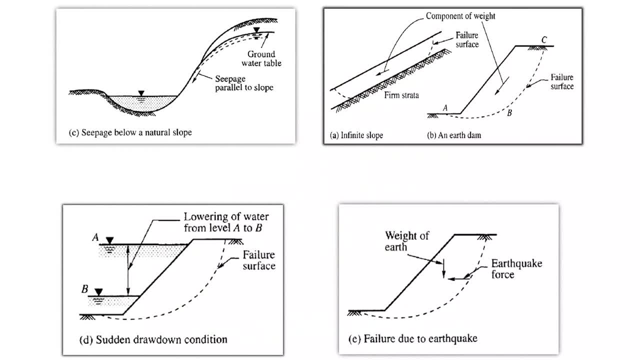 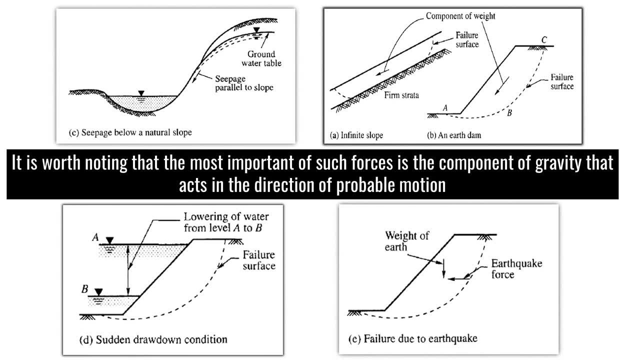 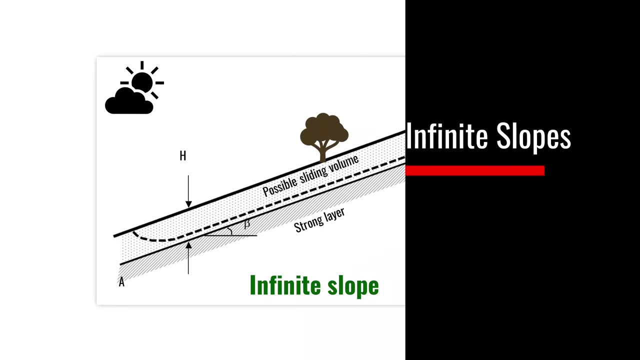 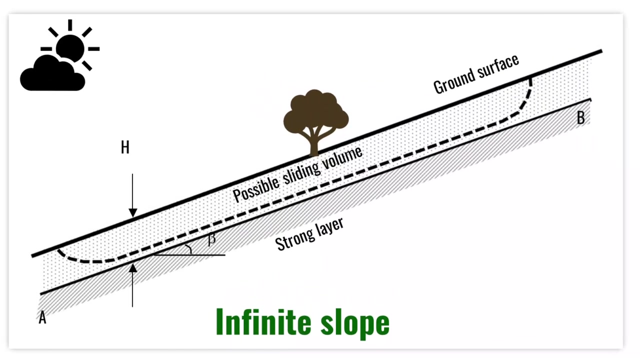 and flows like a liquid. The most important of such forces is the component of gravity that acts in the direction of a probable motion. Let us now talk about infinite slopes. The term infinite slope is used to designate a constant slope of infinite extent. It is usually a slope with adjacent stratum. 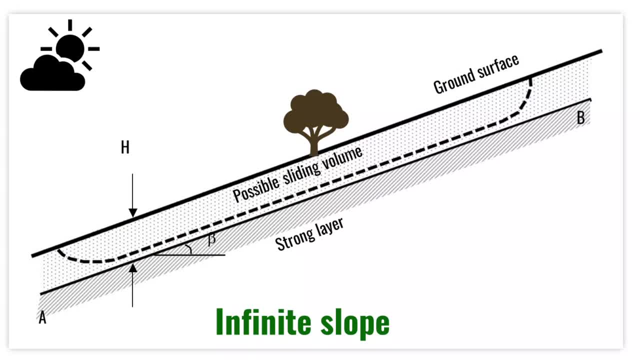 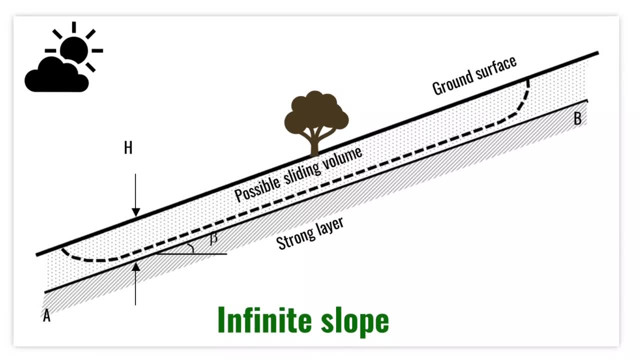 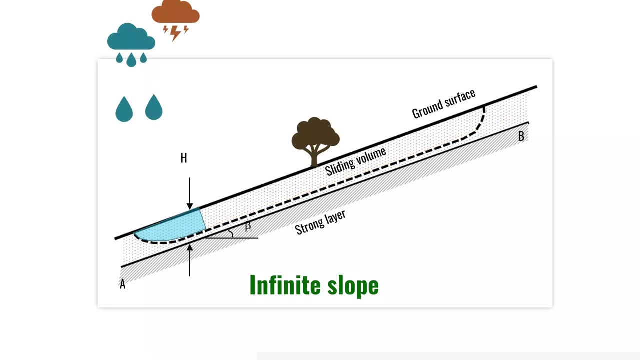 at a relatively shallow depth below surface. The long slope of a face of a mountain is an example of this type. The failure surface is usually a plane parallel to the slope. As we have seen in the Ocean Road, landslide, extreme precipitation can have a significant impact. 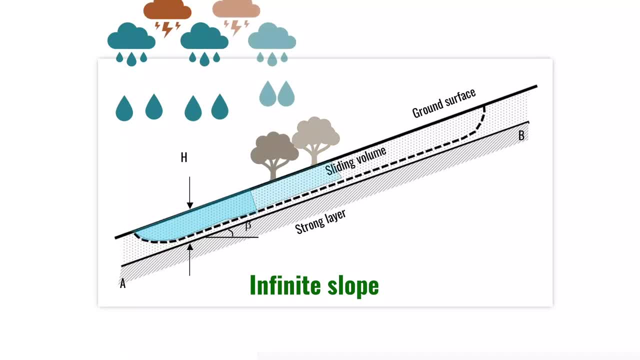 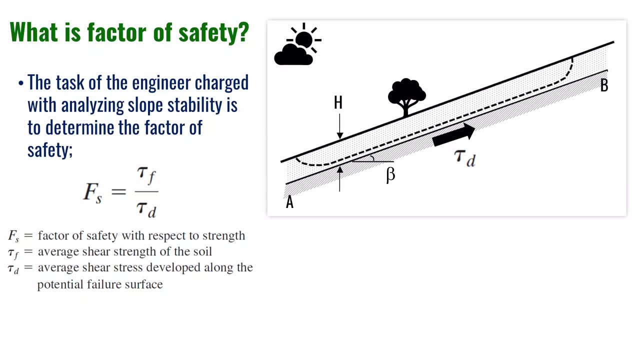 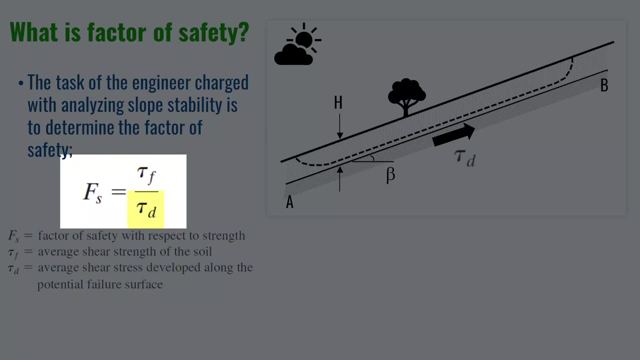 on the shear strength of the soil and can lead to reduction of the factor's safety. So what is factor's safety? Generally, the factor's safety is defined as a ratio between the average shear strength of the soil and the average shear stress developed along the potential failure surface. 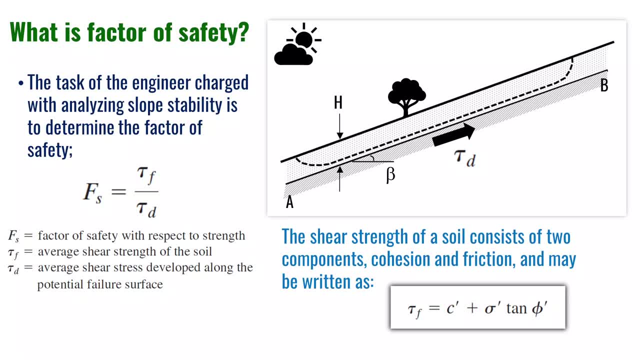 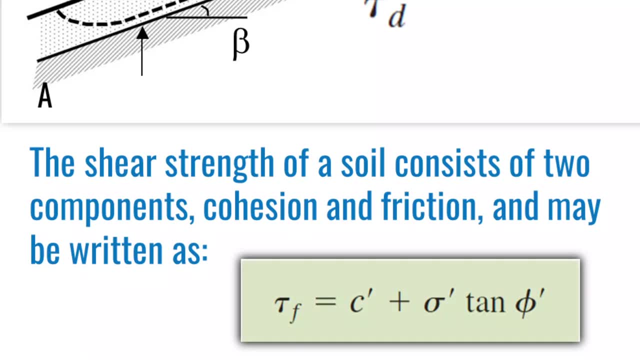 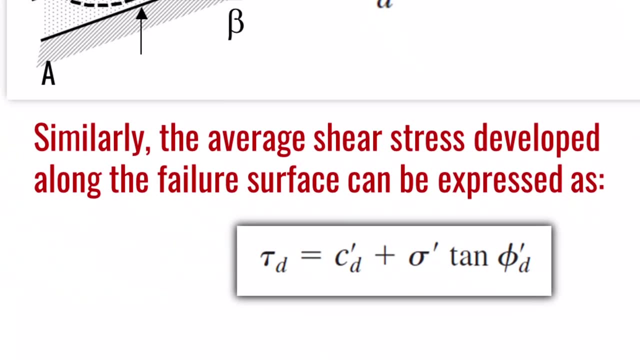 Shear strength can be defined using Mohr-Coulomb failure criteria, where C and Phi prime are the cohesion and friction angle of the soil. Similarly, the developed shear stress can be expressed using Mohr-Coulomb failure criteria, with C and Phi prime, sub d. 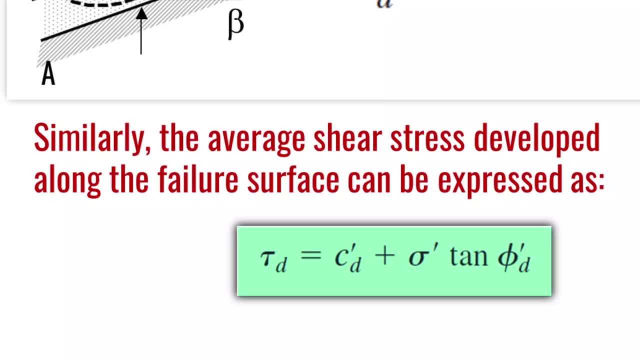 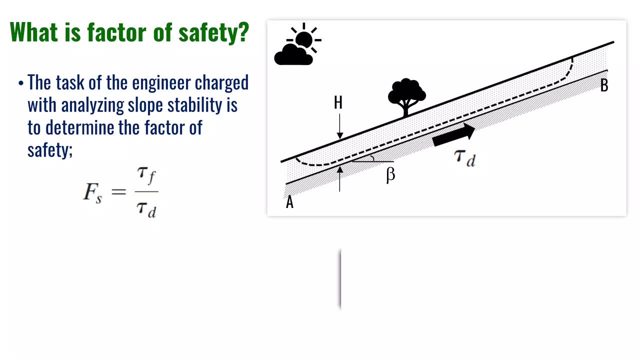 in this case, are the cohesion and friction angle along the failure surface. If you sub the shear strength expression into the factor's safety equation, we get this expression here. When the factor's safety is equal to 1, the slope is in a state of impending failure. 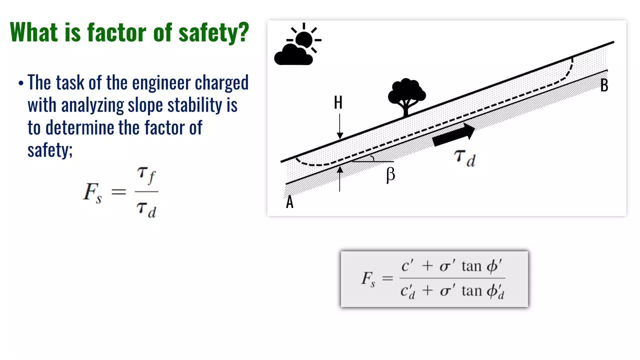 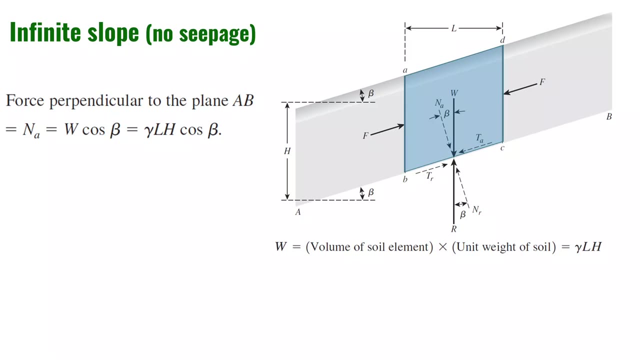 Generally, a value of at least 1.5 for the factor's safety with respect to strength is acceptable for the design of a stable slope. Let us start with the case of an infinite slope shown here, Assuming that the pore pressure is 0,. 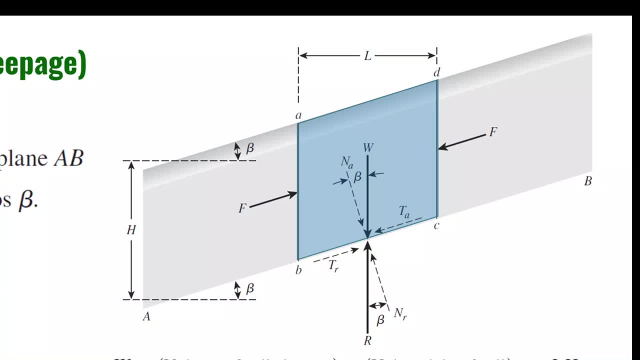 we will evaluate the factor's safety against a possible slope failure along a plane located at a depth below the ground surface. If we consider a slope element that has a unit length normal to the plane of the section, the force that act on the faces are equal and opposite. 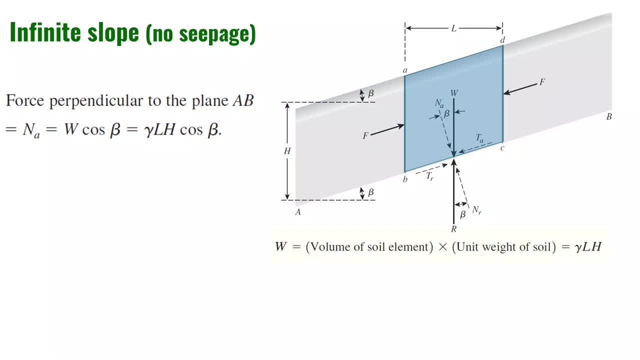 and therefore may be ignored. The weight of the soil element is expressed here as the element volume times unit weight of the soil. The weight W can be resolved into two components: a force normal to the plane AB and a force parallel to the plane AB. 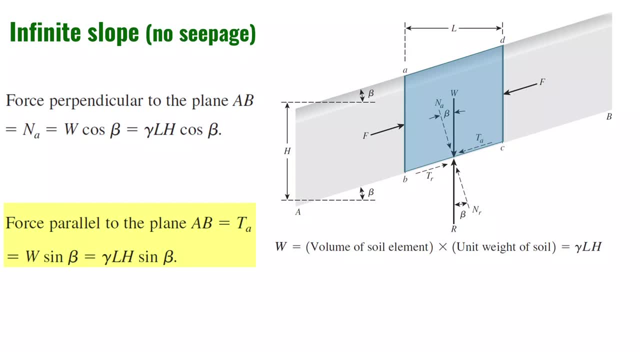 Note that this is the force that tends to cause the slip along the plane. If you divide T sub A and N sub A by the area of the base, which is basically L over cos beta, you get the normal and shear stresses that you need for more Coulomb criteria. 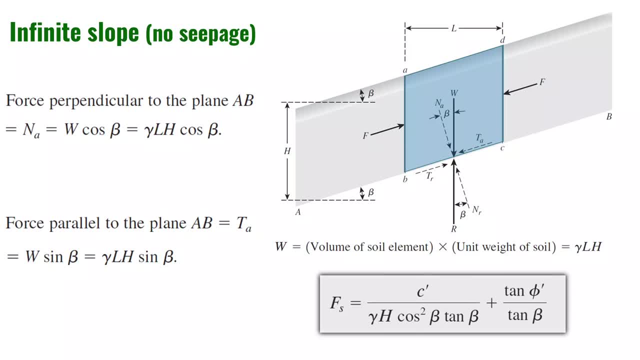 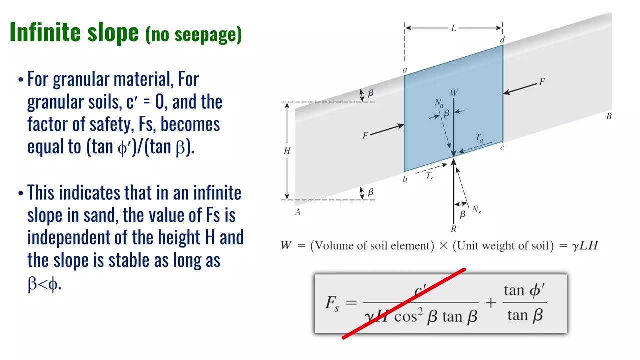 and you will end up with this expression for the factor's safety. For granular material, the cohesion would be 0 and the factor's safety becomes equal to tangent, the friction angle, divided by tangent, the slope angle. This indicates that for an infinite slope in sand, 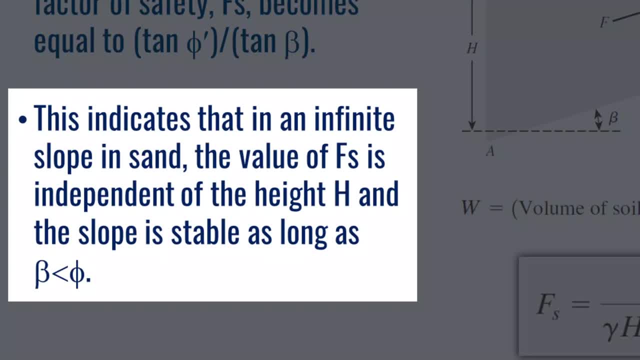 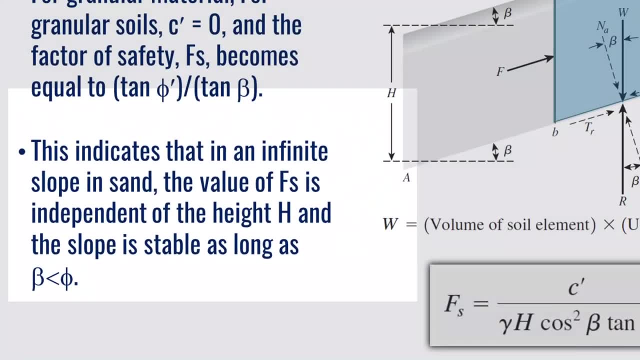 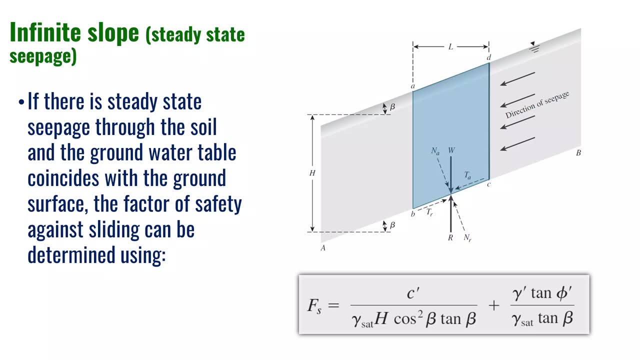 the value of the factor's safety is independent of the height h and the slope would be stable as long as beta is less than phi. You may follow the same approach for the case of steady seepage and you get a similar expression for the factor's safety. 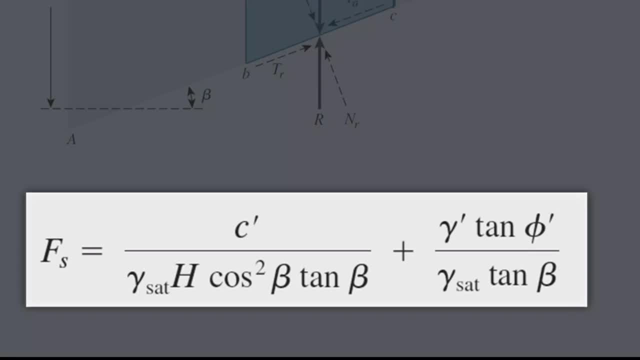 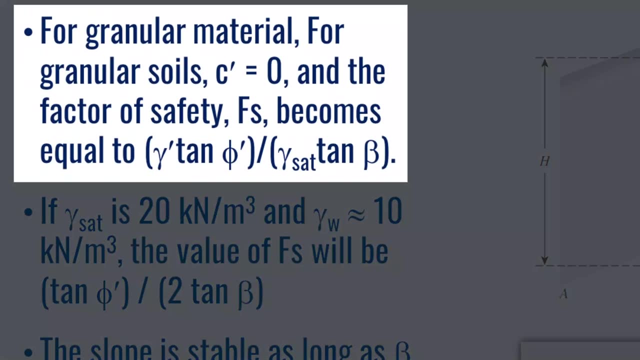 which in this case includes the saturated as well as the buoyant unit weight of the soil For granular material. in this steady state, seepage condition C prime would be 0. The factor's safety would become equal to gamma prime. tangent friction angle prime. 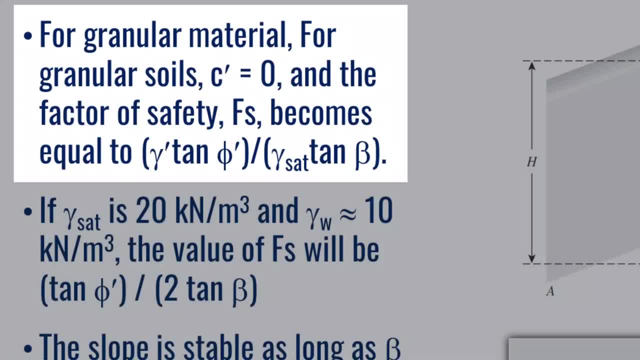 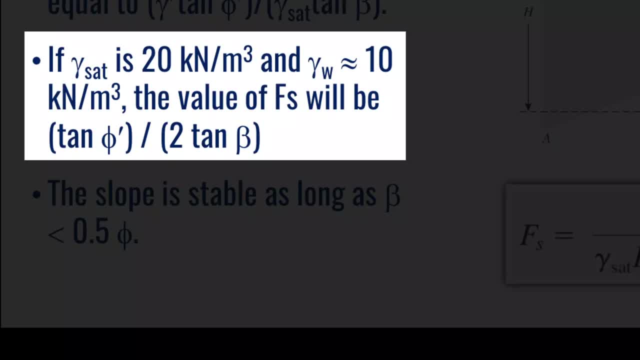 divided by gamma saturated tangent slope angle beta. If the saturated unit weight is taken as 20 kN per cubic meter and unit weight of water is taken as 10, the value of the factor's safety will be tangent friction angle divided by twice tangent the slope angle. 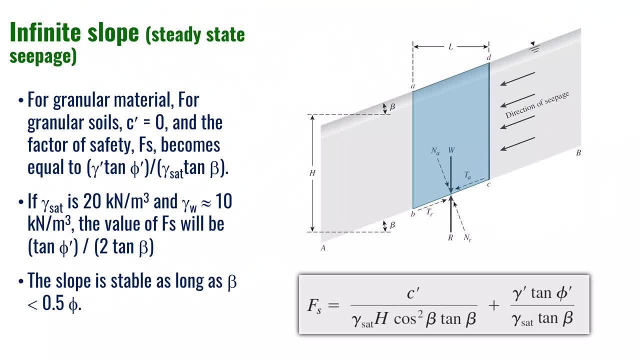 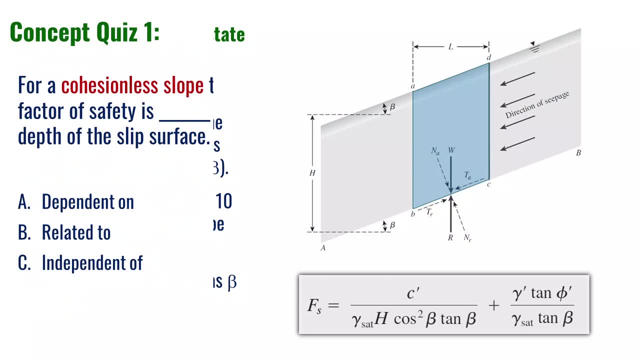 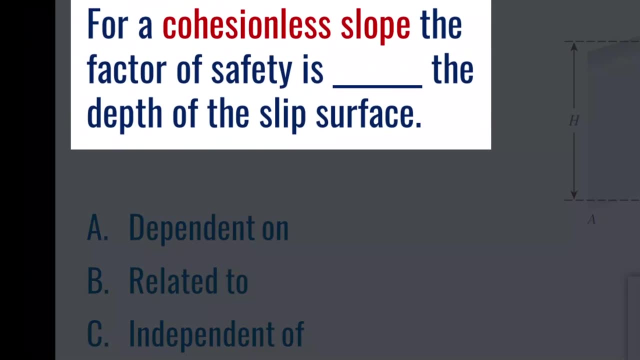 So in this case the slope would be stable as long as beta is less than one half or 0.5 the friction angle. Let's think about this quiz together here. The quiz reads: for a cohesionless slope, the factor's safety is blank. 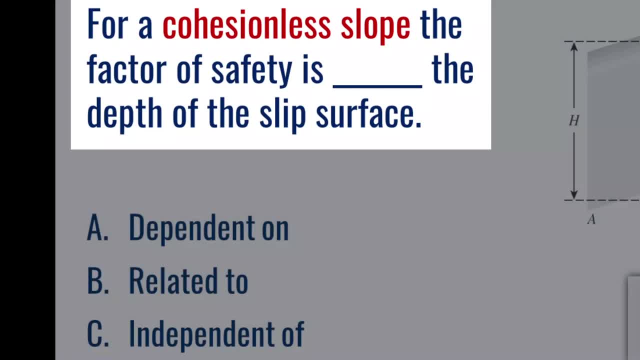 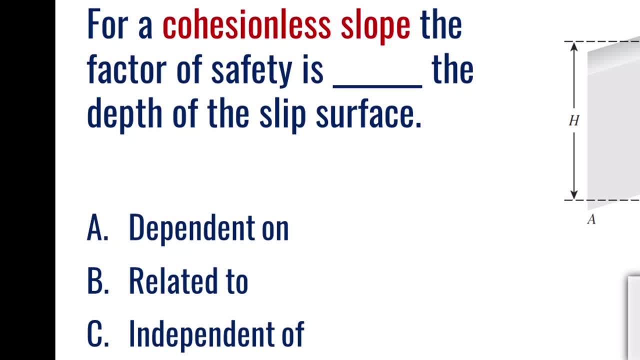 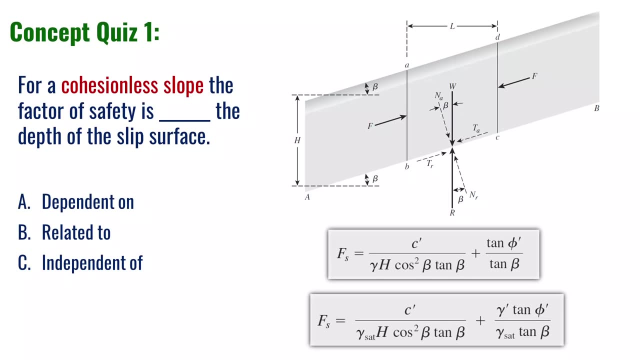 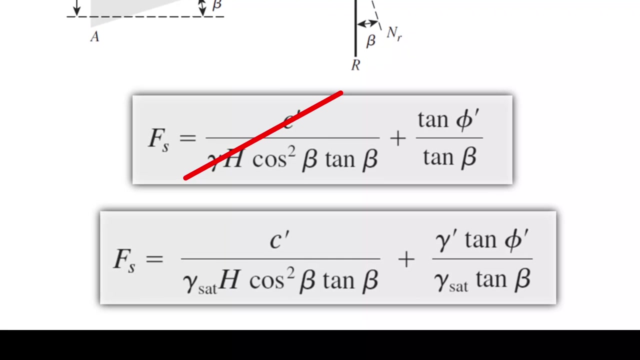 the depth of the slip surface. The options here are dependent on or related to or independent of, So let's look at the factor's safety equation we have here. If cohesion is 0,, the first term will cancel out and we are only left with the second term. 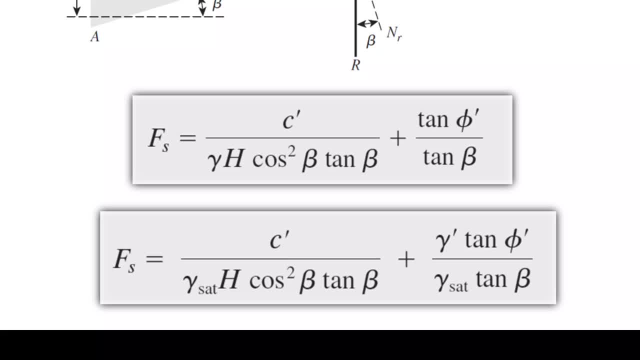 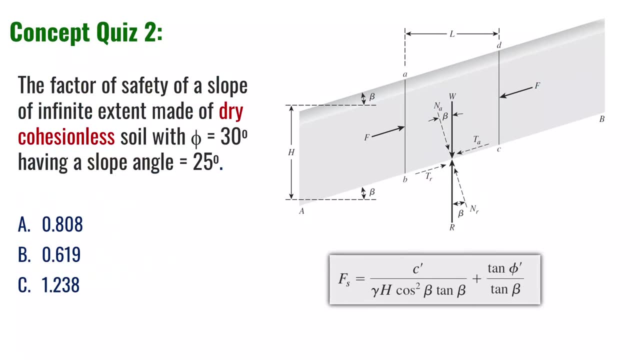 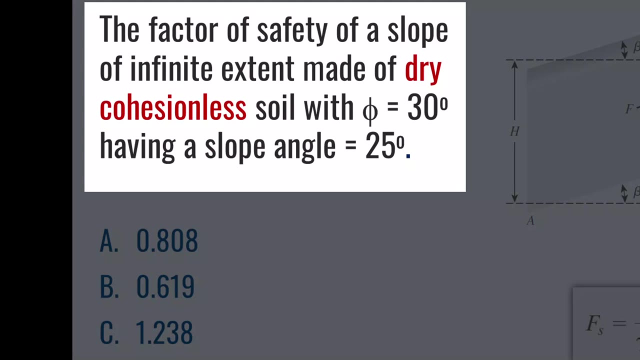 It is obvious that in both cases the factor's safety is independent of the depth of the failure surface. Let's do some simple math here. This quiz reads: the factor's safety of a slope of infinite extent made in dry, cohesionless soil with friction angle of 30 degrees. 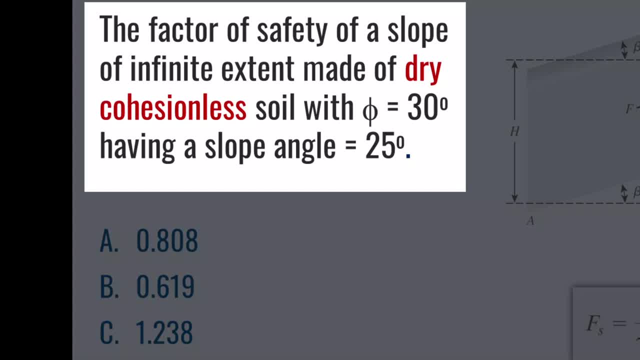 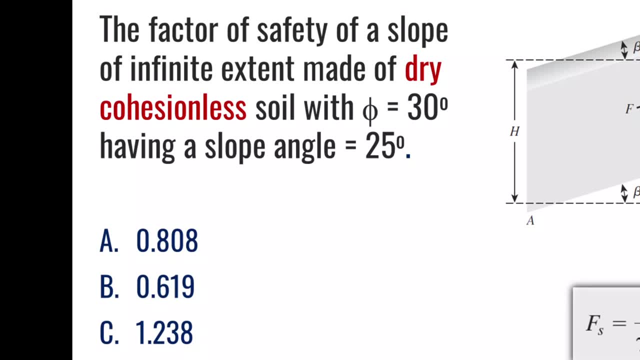 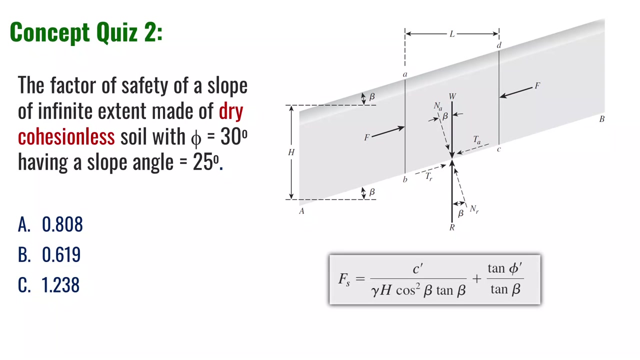 slope angle of 25 degrees would be A 0.808, B 0.619 and C 0.5.. And C 1.238.. If you choose C tangent 30 over tangent 25 or 1.238,, 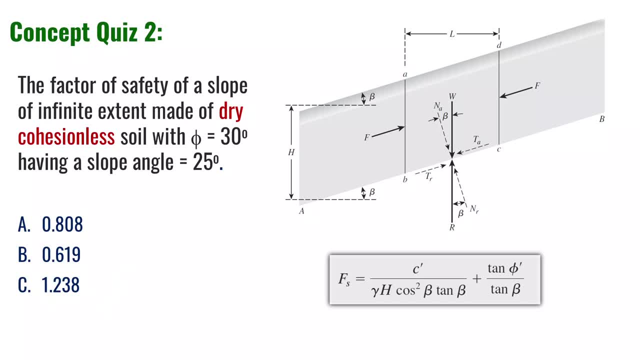 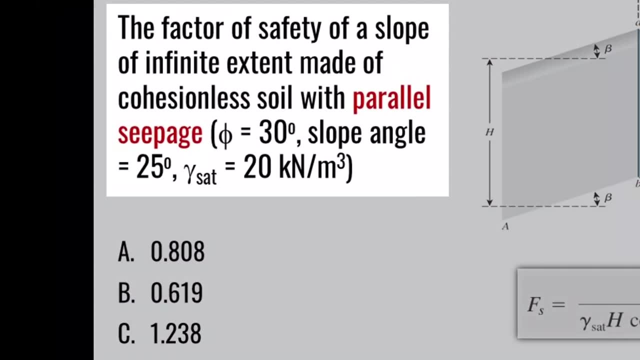 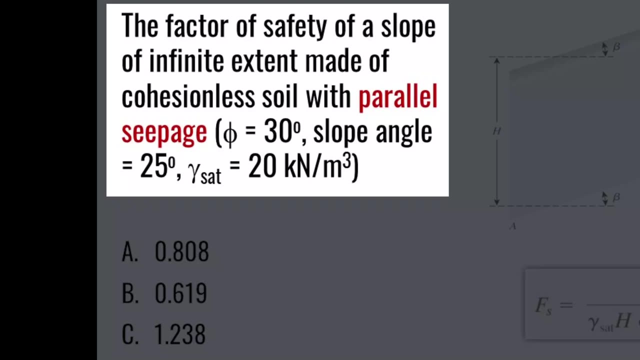 you picked the right answer. One more quiz before we go through some examples: The factor's safety of a slope of infinite extent made of cohesionless soil with parallel seepage, with friction angle of 30 degrees again and slope angle of 25 degrees. 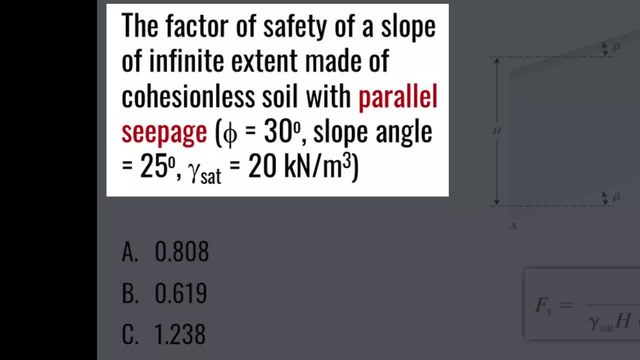 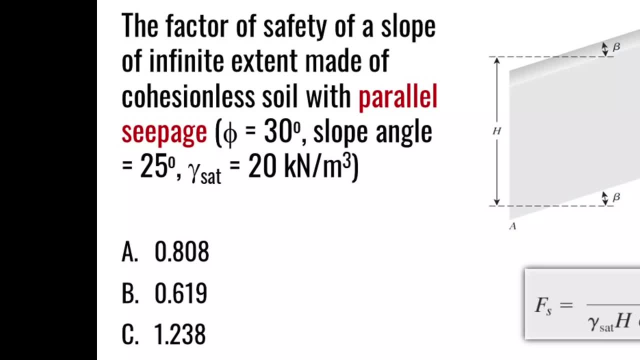 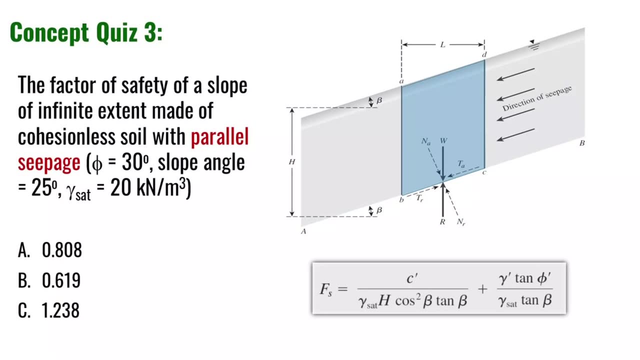 and gamma sat of 20 kN per cubic meter is A 0.808, B 0.619 and C 1.238.. If you choose B 0.619, you got the right answer. Remember that the ratio gamma prime. 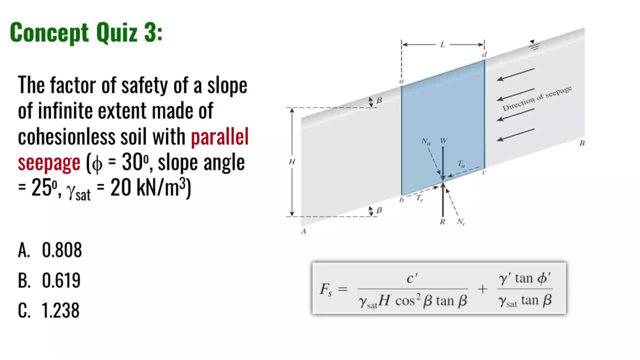 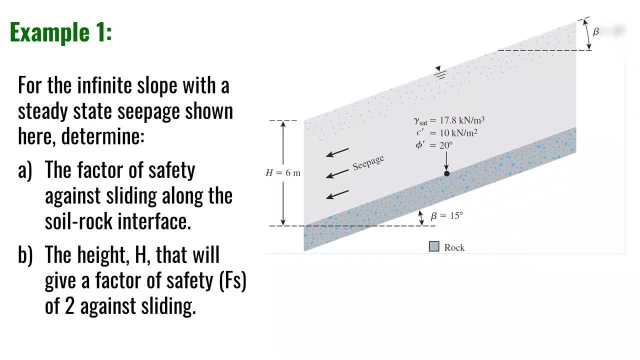 over gamma sat. here is almost one half, And therefore we expect a safety factor of half of that obtained for the dry case. Let's go through this first example here. So we have a 60 meter high slope over bedrock that is making 15 degrees with the horizontal. 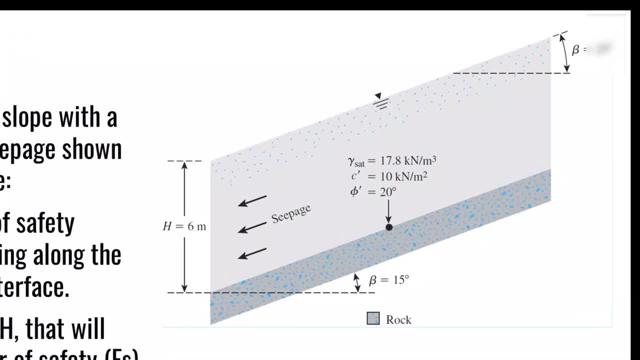 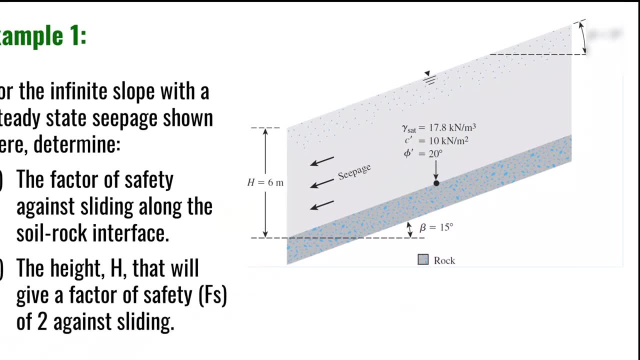 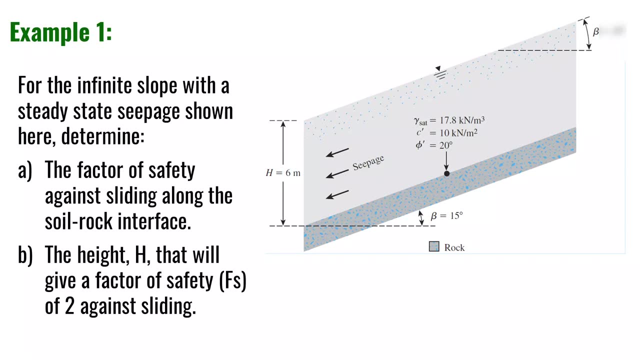 The soil has effective cohesion of 10 kPa and effective friction angle of 20 degrees For the condition of parallel seepage. A- find the factor's safety against sliding along the rock surface And then B find the height H that gives a factor's safety of 2 against sliding. 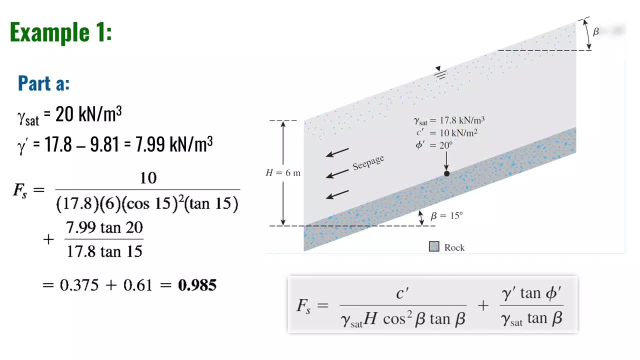 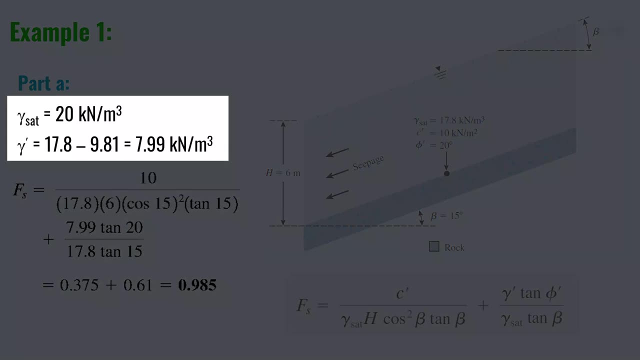 So let's start by writing the equation for the factor's safety for the case of parallel seepage. So since we're dealing with C phi material, in this case, both terms of the equation will be used, Given the saturated unit weight. 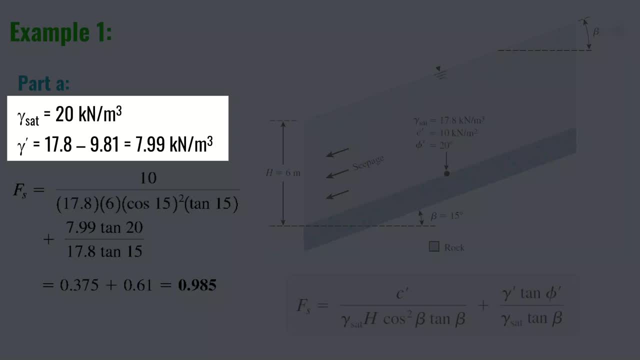 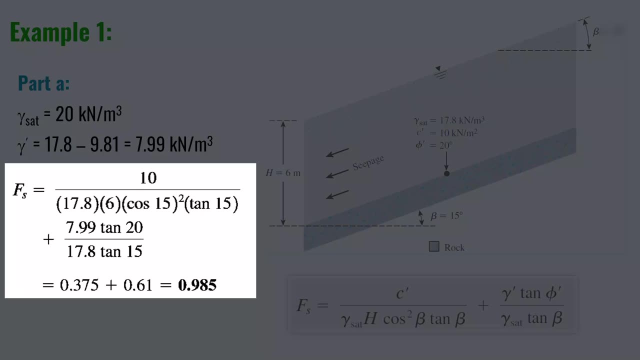 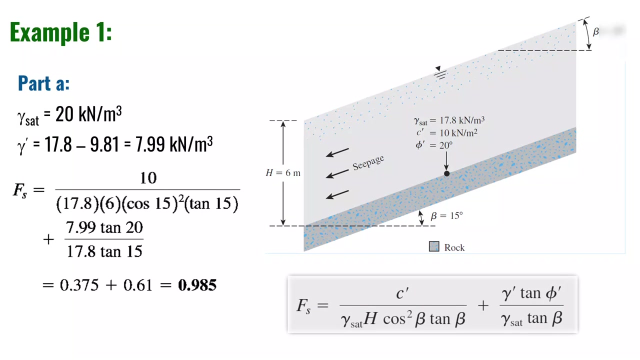 we can find the buoyant unit, weights, and plug the values in the equation And adding up both terms, we can get a factor's safety, in this case, of less than 1. This is definitely unacceptable And that's why the second part of the question. 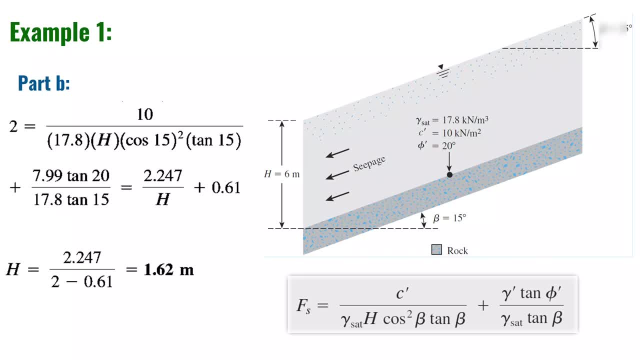 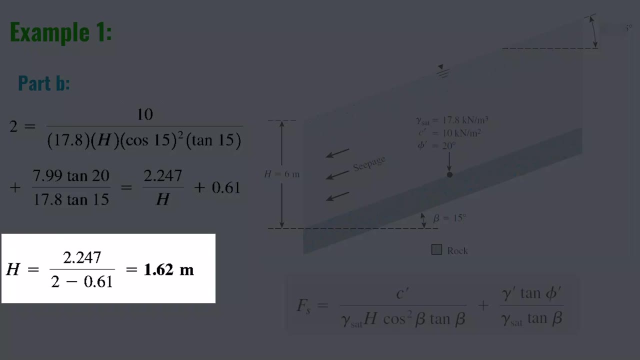 asks for this slope height that will correspond to a factor's safety of 2.. Now the factor's safety is known and the same equation can be used with H as unknown. If you solve for H, you get a maximum height of the slope that corresponds. 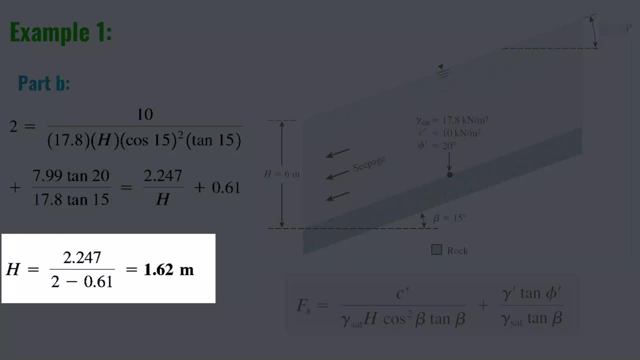 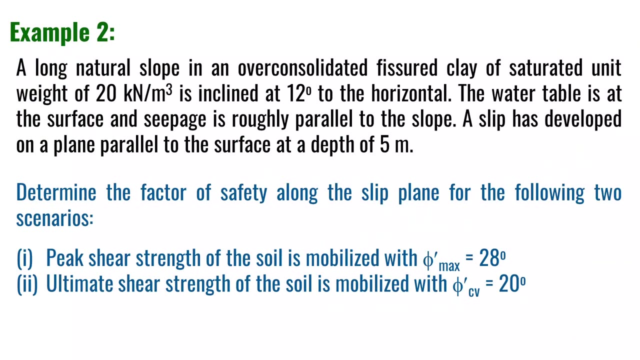 to a factor's safety of 2, that is, 1.62 m, which is again significantly lower than the original slope height. The last example I would like to share with you here reads: a long natural slope in an over-concentrated fissured clay. 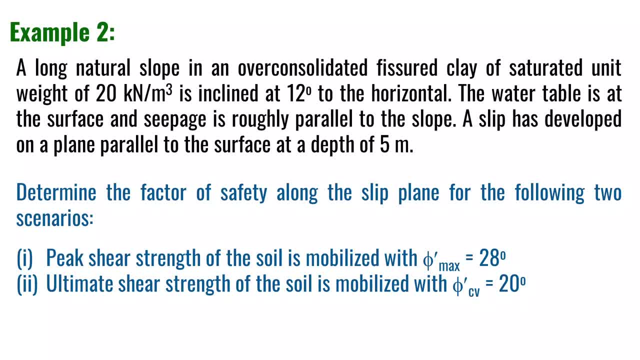 of saturated unit weight of 20 is inclined at 12 degrees to the horizontal. The water table is at the surface and seepage is roughly parallel to the slope. A slip has developed on a plane parallel to the surface at a depth of 5 m. 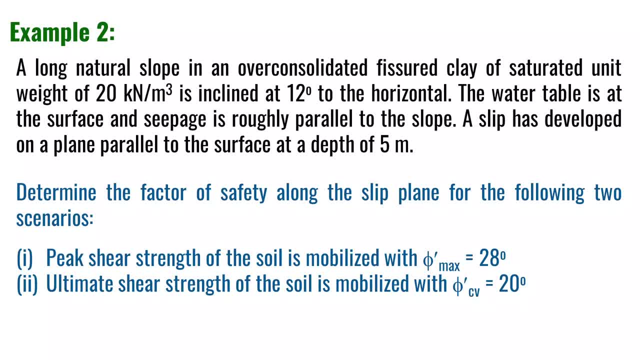 Determine the factor's safety along the slip plane for the following two scenarios: First, peak shear strength of the soil is mobilized with phi prime maximum of 28 degrees. And second, ultimate shear strength of the soil is mobilized with constant volume friction angle. 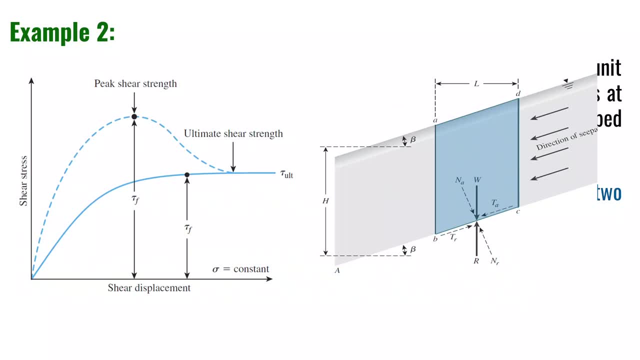 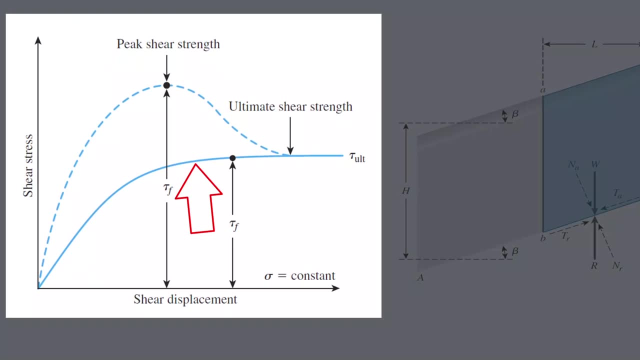 of 20 degrees. As explained in episode 2 of this series, loose sand and normally concentrated clays can exhibit strain hardening behavior under shear, whereas dense sand and over-concentrated clays exhibit strain softening behavior with two shear strength values.